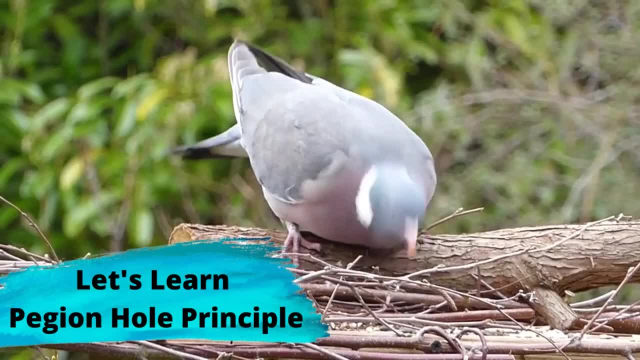 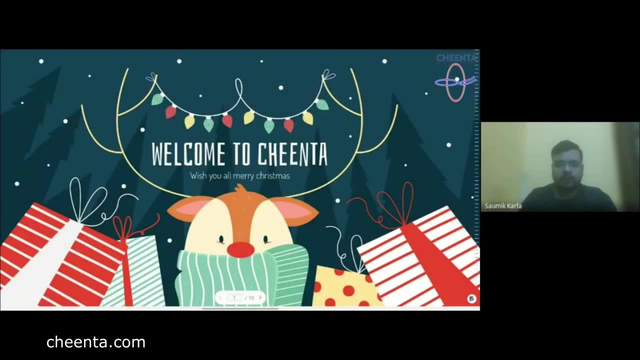 Hello, welcome to Chinta's YouTube channel. I am Tomik Karfa, one of the faculties of Chinta, So today our topic of discussion will be a problem based on Pigeonal Principle. Basically, this problem is based on two topics. Let me share the problem first, then we'll discuss about the. 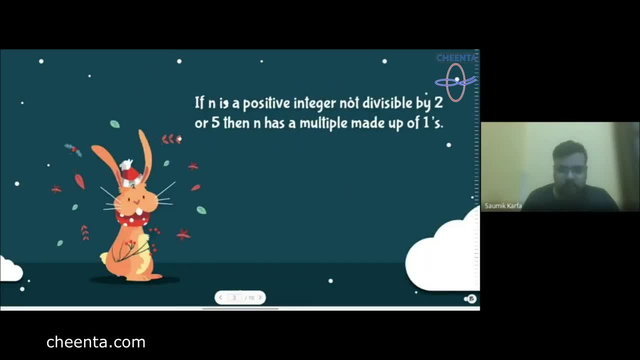 topics Here. if you can read the problem: if n is a positive integer not divisible by 2 or 5, then n has a multiple made up of 1s only. So at the first glance the problem seems to be. 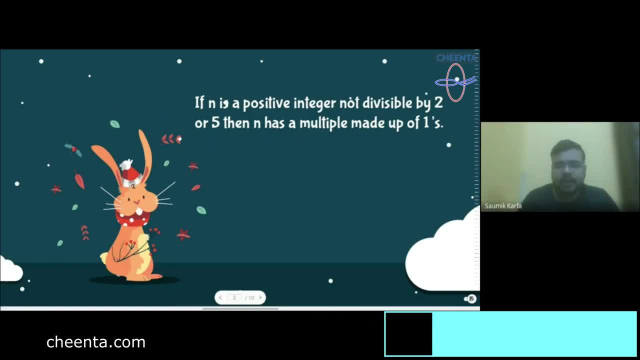 on the topic of divisibility. but basically we'll take help of Pigeonal Principle to solve this problem. Before we start, you can give it a try, So you can pause the video and try to solve this problem. Okay, So now, before we start solving this problem, we will try to see. 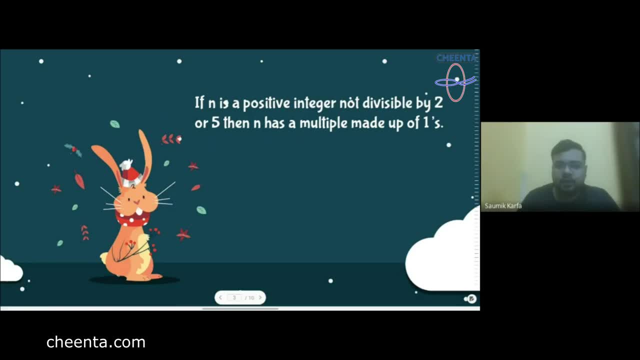 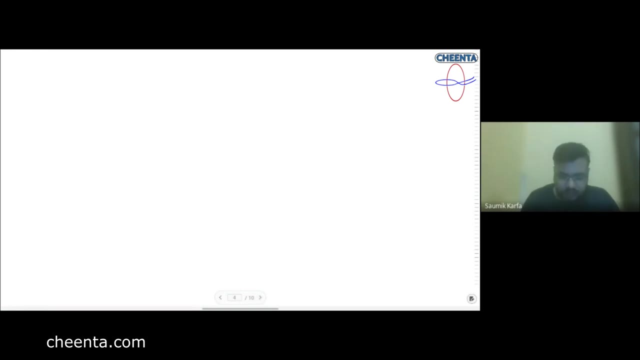 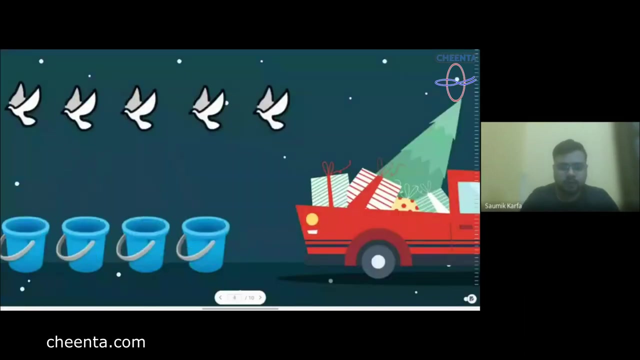 what Pigeonal Principle is. Okay, So Pigeonal Principle is a very simple, yet a very strong principle that we can use to solve a vast range of problems. What is that? Let us see. Okay, If you have Just hold on a moment, Yeah. So if you have, let's say, 4 buckets with you, 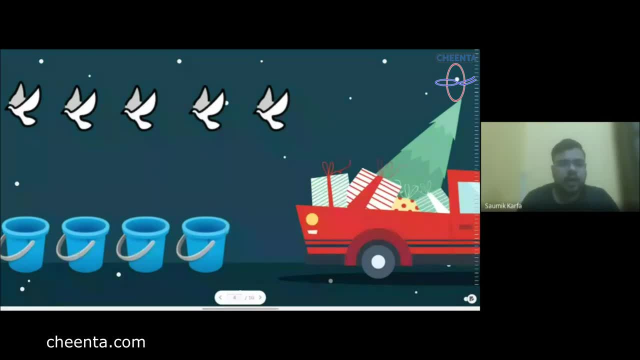 and 5 pigeons and you are asked to accommodate those pigeons in these buckets. Okay, So how you can do that- And the rule is you can put multiple pigeons in one bucket. So there are many ways to do so. You can put all 5 pigeons in one bucket, or you can put 4 in one, 1 in another. Okay, 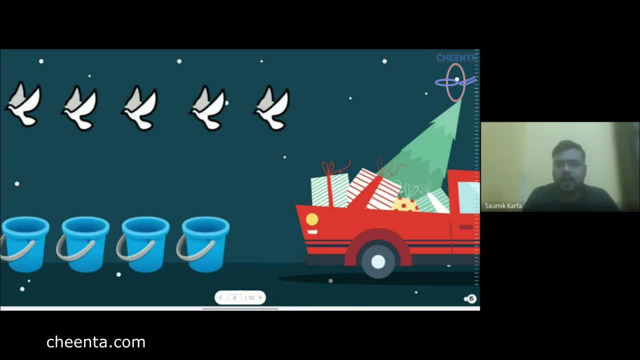 Let the other buckets empty And in such way you can get many ways to put these pigeons in these buckets. And the best possible way that can be is like this: You can put 4 pigeons each on one bucket. Then you will be left with 1 pigeon only When you will try to put that 5th pigeon. 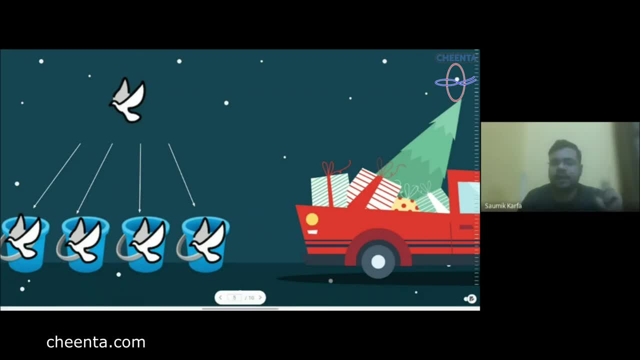 in one of these buckets, then at least 1 bucket will contain more than 1 pigeon. Okay, That is it. Now you may think that how we can use or solve a problem because this is very simple. Okay, That is the interesting thing about P-general principle. So we see how we can solve that. 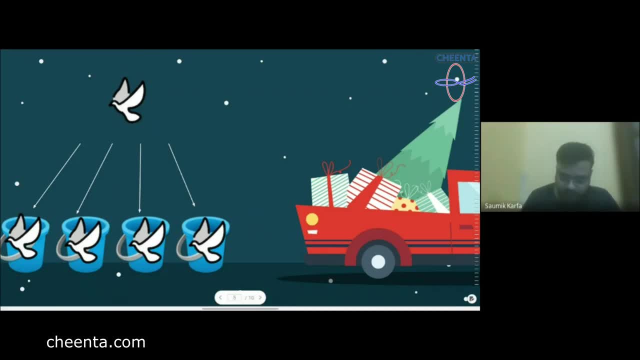 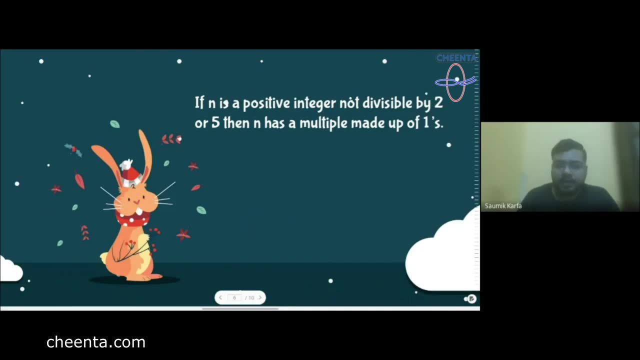 problem that we have seen earlier using P-general principle. Okay, So let's get back to the problem again. Here is it. So n is a positive integer not divisible by 2 or 5. Then n has a multiple made up of only 1.. Like there will be a multiple of n where all the digits 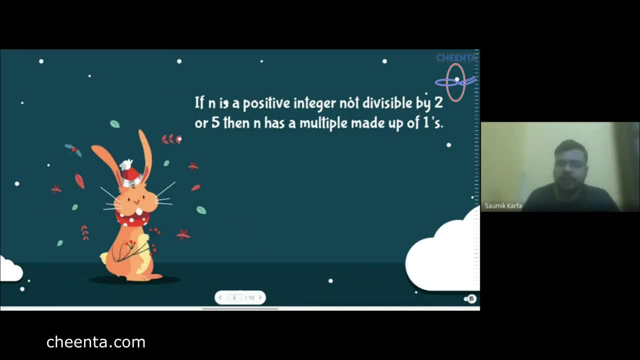 of that number will be 1.. Okay, We don't know the number of digits, but, whatever, how many digits are there? all of them are 1 only. Okay. First of all, we need to notice one thing: that n is not a multiple of 2 or 5. That means n is not a multiple of 10.. Okay, That is the main thing. 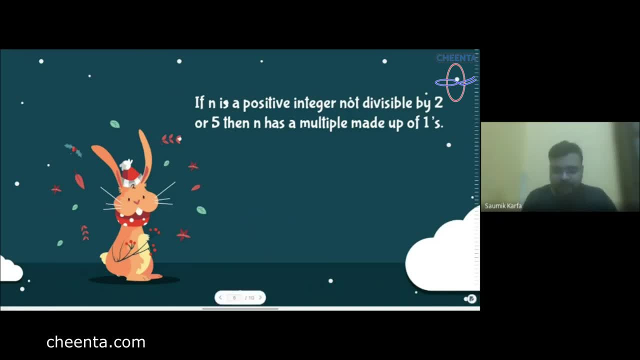 we have to know Now what we will do. We will consider a list of numbers. Those are, let's say, 1, then 11, then 111, then 41.. Okay, And so. okay, So n-th term of the sequence, we can. 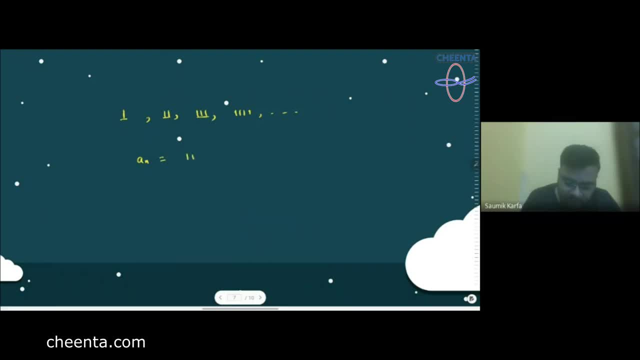 say, if we denote it with a n, that will contain n 1s in it. Sorry, That will contain n 1 in it. Okay, So there are n digits. All are 1.. Okay, Now think if one of these numbers 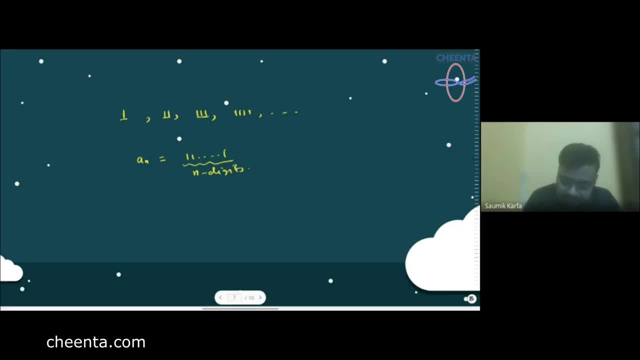 are there. So how many numbers we have considered? actually, We have considered n numbers. The last number here is that n. Okay, The last number here is n, that n. So we have considered n numbers here and all of them are made up of 1.. So if one of these numbers from this list is a multiple of, 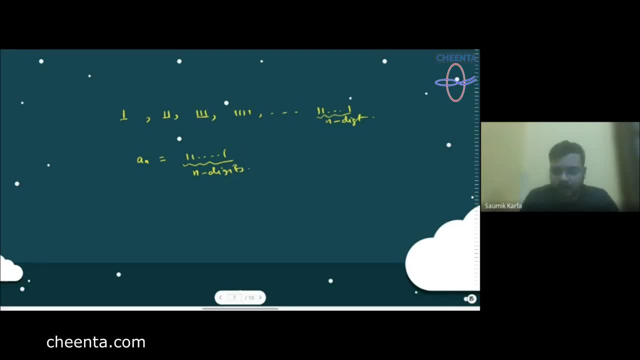 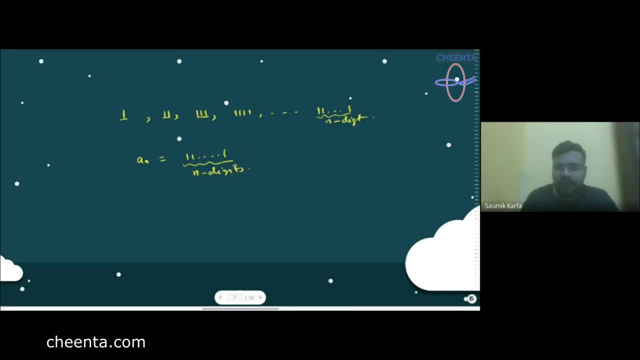 see. Now we need to see a very interesting property of divisibility: that if you divide any positive integer by the number, by any integer n, then the possible remainders that you can get are 0 or 1 or 2 or 3, or all the way up to n minus 1.. Like you can, give it a try, Like you can. 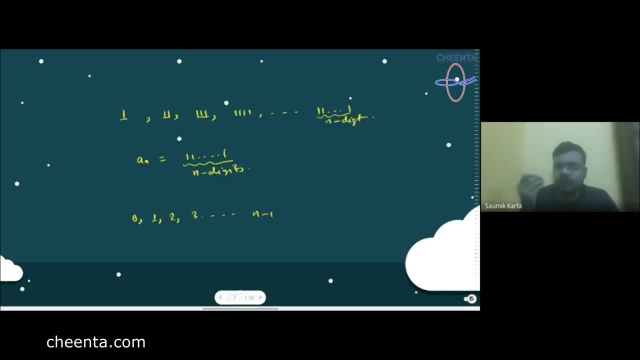 try to divide several numbers, let us say with 3. You will see that you can only get the remainder 0 or 1 or 2, not more than that, Okay. So now, if we try to divide any number by n, 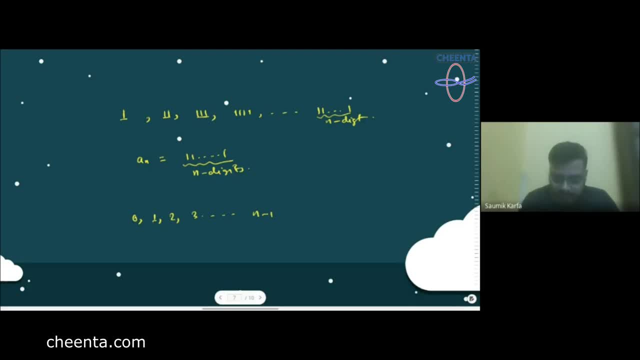 these are the different remainders that we can get. Now, if we try to divide all these numbers by n, we cannot get 0. Why? Because we already considered that none of these numbers are divisible by n, So we should not get 0 as the remainder. So the possibilities of remainders are starting. 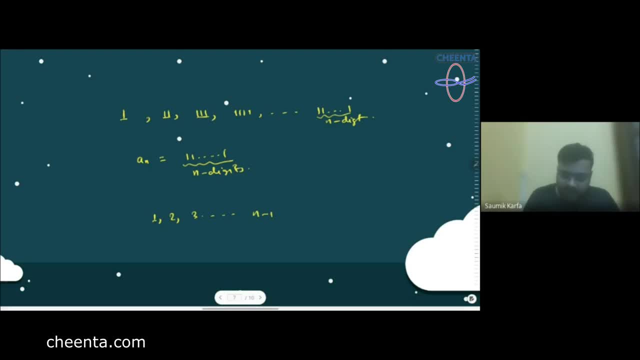 from 1 to n minus 1.. So we should not get 0 as the remainder. So the possibilities of remainders are starting from 1 to n minus 1.. Okay, Now think we have n minus 1 buckets. We have n minus 1. 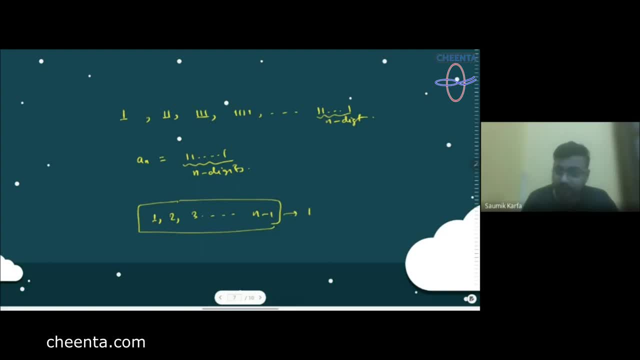 buckets, These are our buckets, or we can call it pigeonholes. Okay, Pigeonholes, So let us call them holes. We have these many holes. All are tagged with these numbers. One hole is tagged with 1, then another with 2,, 3,, 4 and so on up to n minus 1.. And we have n pigeons. Those are. 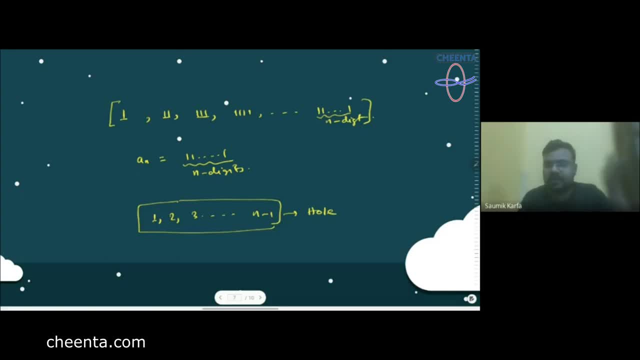 our pigeons. Pigeons are also tagged Like: there is a pigeon called 1., There is a pigeon called 2., There is a pigeon called 11. Then 111, and so on. Okay, Now we will put these pigeons. 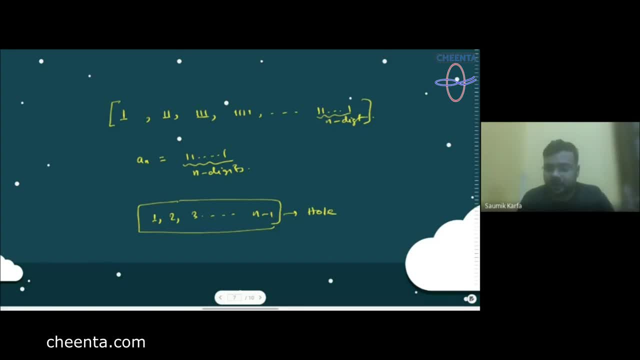 in those buckets according to their remainder. Okay, So let us say, if we divide 1 by n, we should get 1 as the remainder. Okay, That is the possibility that we should get 1 as the remainder. Okay. So we will put this 1 in this bucket called 1.. Okay, If 11 gives. 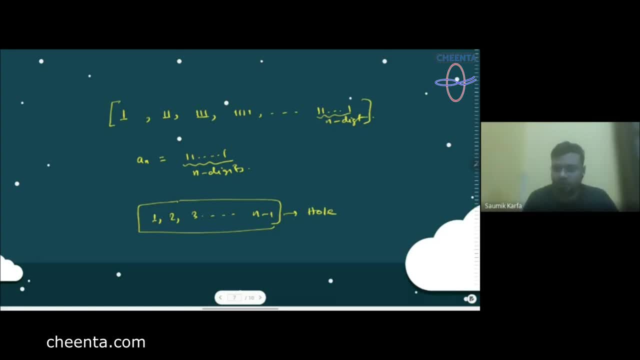 us 2 as the remainder. we will put 11 in bucket 2, and so on. Okay, Now as now, what we are going to do is we are going to put this 1 in this bucket called 1.. Okay, Now as now. 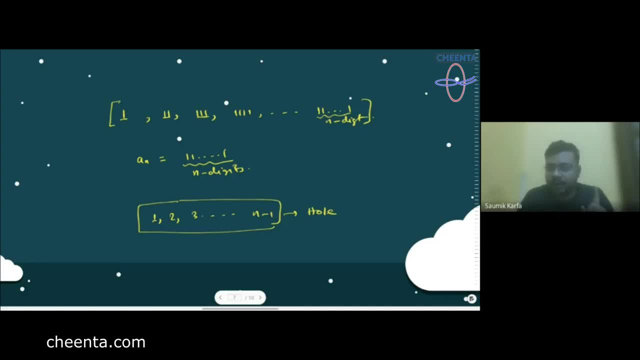 by pigeon principle what we can say: There will be at least one bucket which will contain more than one pigeon, or at least two pigeons will be there, Right, Okay, Let us say those pigeons are a, i and a j. Okay, a, i and a j are the pigeons which are on this in the 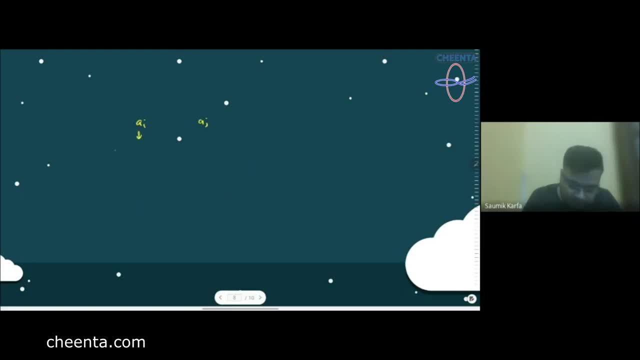 same bucket. Okay. So a i is what? a i is a number made up of i digits and a j is a number made up of i digits. All digits are 1.. Okay, And a j is a number made up of j digits. 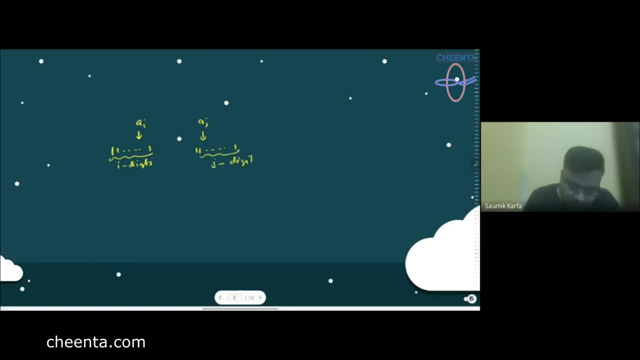 All digits are 1 here. Okay, j digits- All digits are 1 here. Now they are in same bucket. What does that mean? That means they have same remainder when we are trying to divide them by n. That means if you subtract these two numbers, then the resultant number that 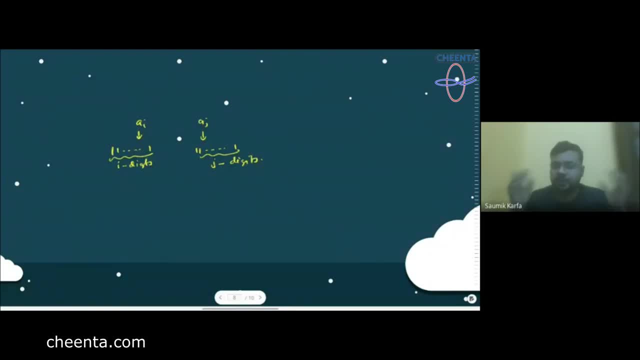 will be a divisible. that will be divisible by n, Isn't that Okay? So let us subtract a i from a j Without any loss of generative. we can say that i is greater than j. That means a i is greater than a j. So let us subtract a j from a i. Okay, So there are. 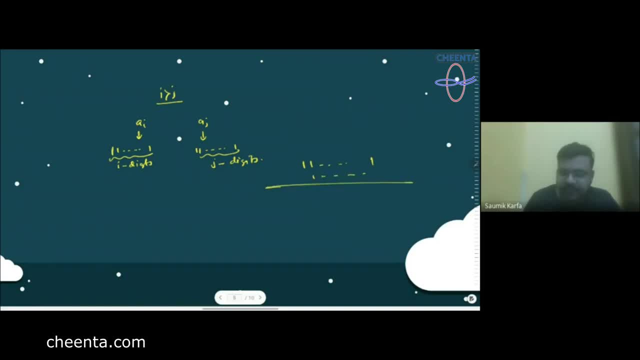 i 1 and there are j 1s. So the resultant number- whatever the number will be that will contain i minus j 1s. There will be i minus j 1 and then remaining j 1s. Okay So. 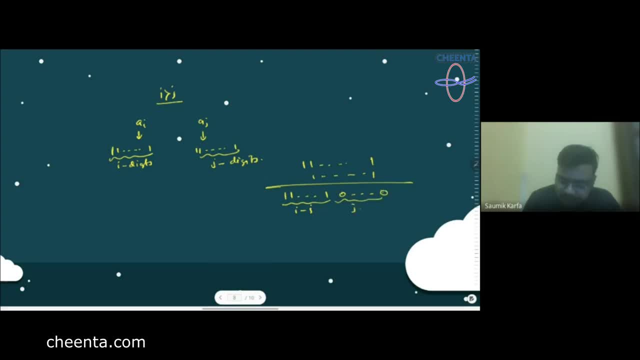 the resultant number, like j digits, will be 0.. Okay, j digits will be 0.. Okay, Now this number can be represented as: i minus j, 1 times 10 to the power j, And we know that n divides this number, Right, n divides this number, Okay. Now think n is not a multiple of 10. 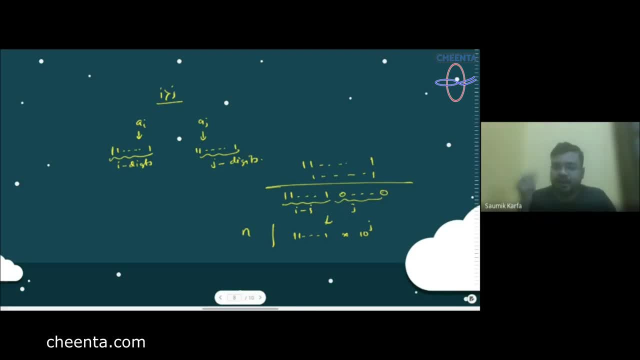 and that gives us: n cannot divide 10 to the power j as well. Okay, n cannot divide 10 to the power j. Okay, So it should not divide any multiples of 10 as well, Right? So any power of 10, that. 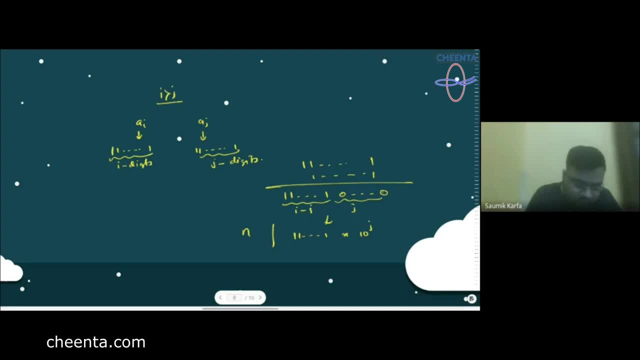 will not be divisible by n, But n divides this total product. n divides this total product, So n must divide this part. then, as n does not divide this 10 to the power, j n must divide this. Okay. So that means this number here: 1, 1, 1, i minus j. 1 containing i minus. 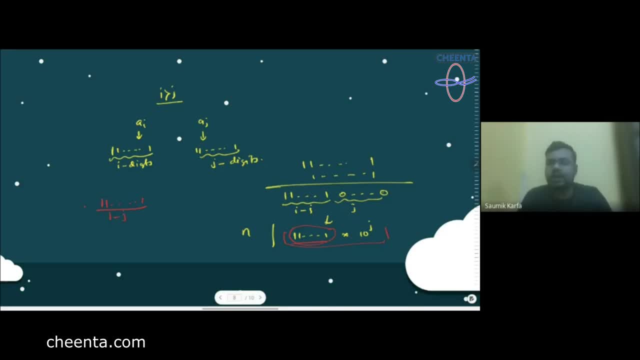 j, 1.. This is the multiple of n, And this multiple contains all digits as 1.. Right, So that proves our problem. I hope you have enjoyed this problem. We will meet again in the next video. By then, keep doing great mathematics. Bye. 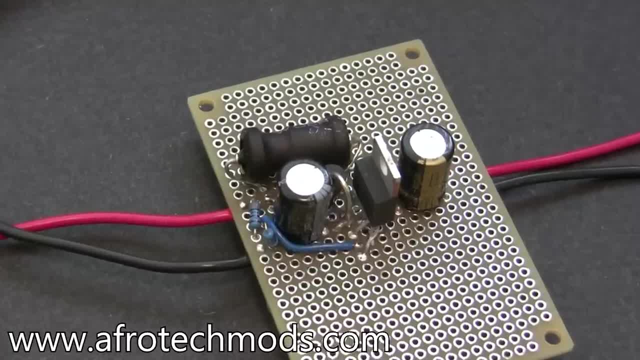 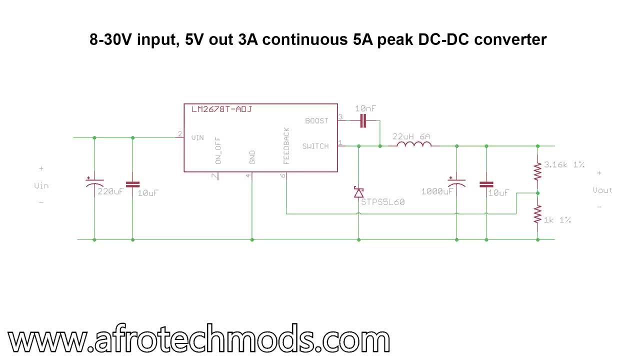 Today I'm going to teach you about buck converters and show you how to make a switch mode power supply that can work with input voltages between 8 and 30 volts, and it steps the output down to 5 volts. It can supply 3 amps continuously and it can handle peak currents of up to 5. 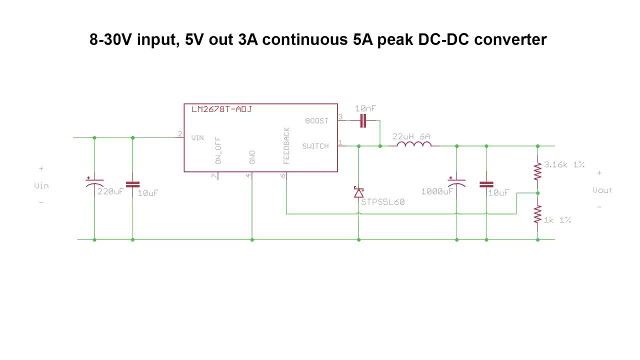 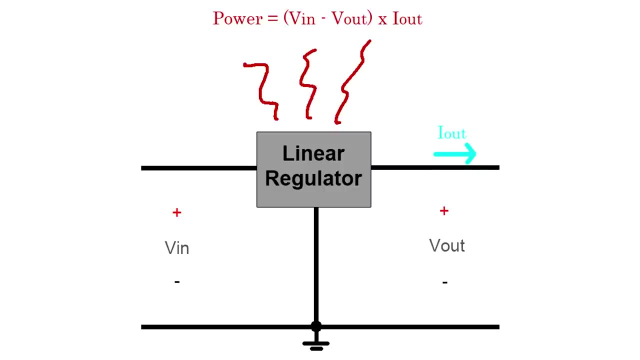 amps for several minutes. Let's start with why we need switch mode power supplies in the first place. In previous videos I talked about linear voltage regulators like the LM7805 and LM317.. These are really easy to use, but they're very inefficient at high voltages, For example, if you try to power. 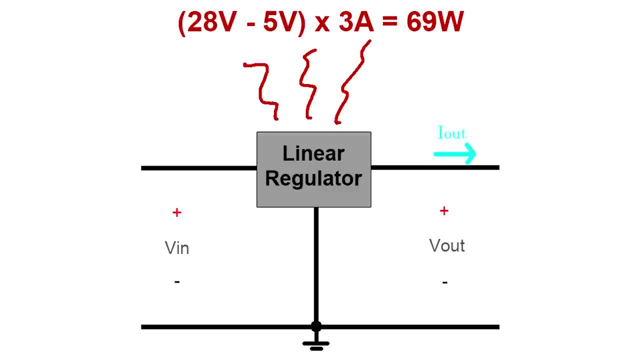 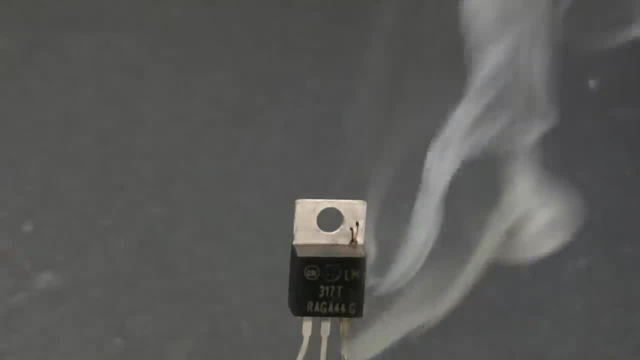 a linear voltage regulator with 28 volts and had 5 volts and 3 amps on the output, you'd end up with 69 watts of heat produced and that might cause a few problems with your circuit. For high powered projects, you want to be using what is called a switch mode power supply. 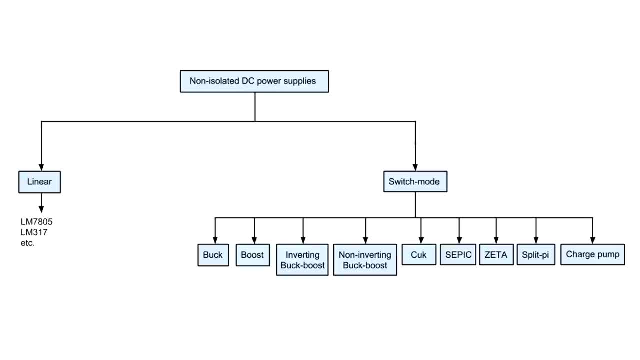 There are many different types of switch mode power supplies that can get you from one voltage to another, but today we're going to talk about buck converters, which is a type of supply that can work with input voltages between 8 and 30 volts. Let's start with an input voltage of 10 volts and let's put a switch in series with it. 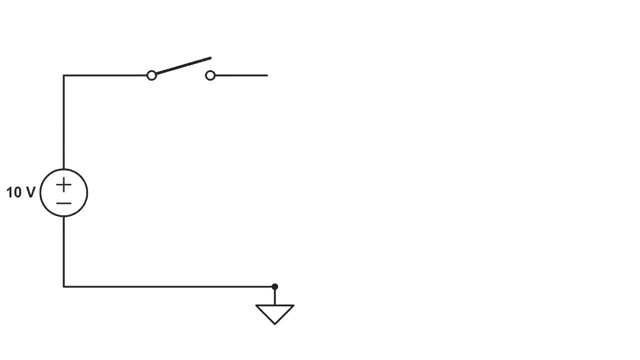 It doesn't matter what the switch is. It could be a bipolar transistor, a MOSFET or even a crackhead mashing, a mechanical switch. For efficiency reasons, you should use a MOSFET, but let's just use a generic switch symbol for now. Next, let's control the switch with. 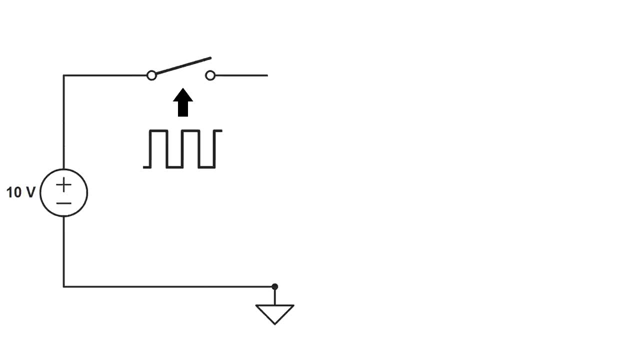 a high frequency pulse width modulated signal with a duty cycle of 50%. This will give us a square wave that's 10 volts high and a pulse width modulated signal with a duty cycle of 50%. This will give us a square wave that's 10 volts high and a pulse width modulated.